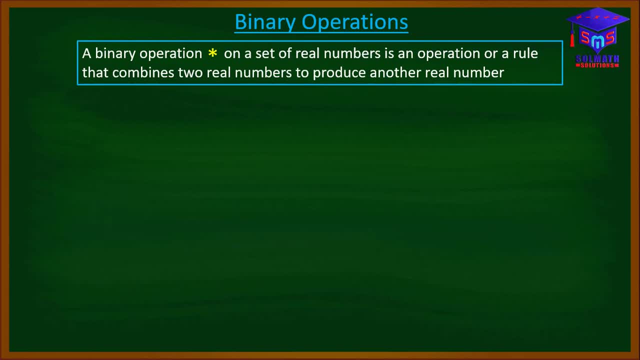 A binary operation star on a set of real numbers is an operation or a rule that combines two real numbers to produce another real number. What we are trying to say is that, assuming we have two real numbers, let's say A and B, we can combine these two real numbers with an operation- let's say star, to produce another real number, C. 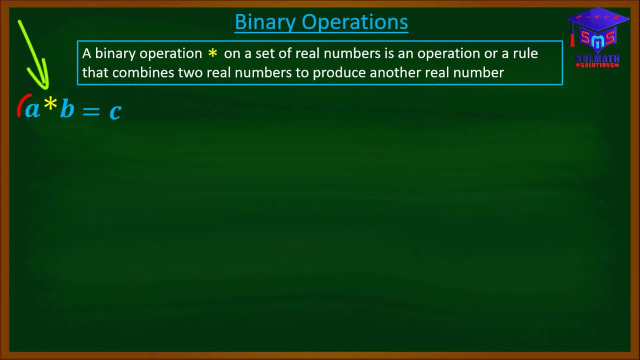 So the operation we use to combine these two real numbers is called a binary operation. So the operation we use to combine these two real numbers, A and B, is what we call the binary operation, And that operation can be addition, subtraction, multiplication, division or any other binary operation. 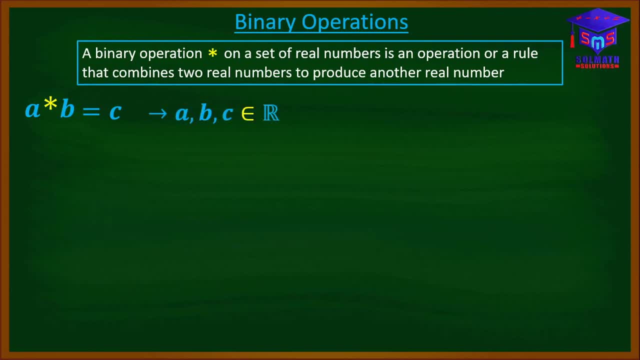 And so A, B and C are all real numbers. For example, if you have 3 plus 2, the two real numbers are 3 and 2.. And then we are combining them with the addition operation to get what? 5,, which is also a real number. 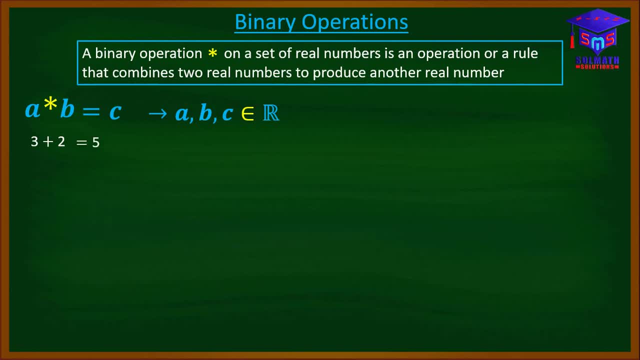 And then we are combining them with the addition operation to get what? 5,, which is also a real number. So in this case, our binary operation is what Addition Over. here too we have two real numbers, 4 and 8, which are being combined with an operation subtraction to produce another real number, negative 4.. 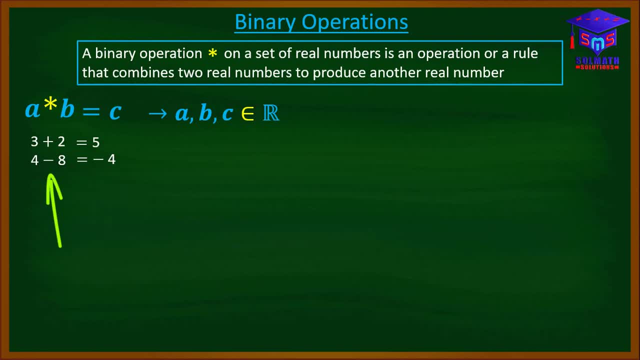 And so the binary operation in this case is what Subtraction. Over here too, the binary operation is what Multiplication, And then, over here too, the binary operation is division. And so these are the basic binary operations, But in the case where we want to perform an operation which involves two or more of these basic binary operations, 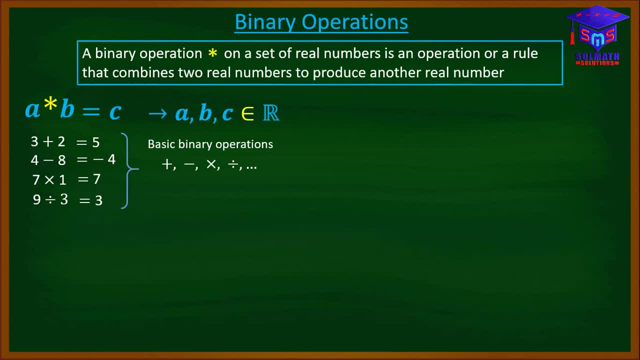 then we have to use a defined binary operation, And so other binary operations can be defined, as A star B is equal to A plus, B, minus. what A B? In this case, we are combining what Addition, subtraction and what Multiplication. 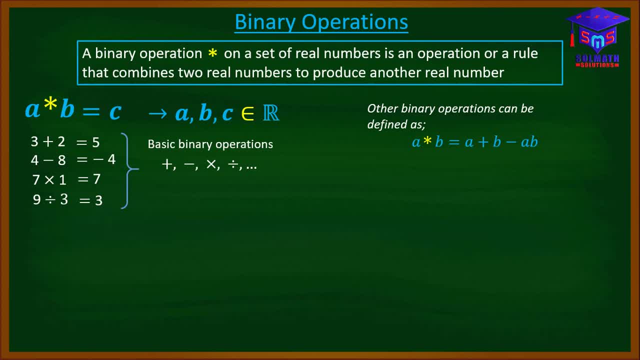 So therefore, we have to use a defined operation. So in this case, we are combining these two real numbers, A and B, with the operation star, And so our binary operation in this case is what Star? And then all this you see over here is the definition of the operation. 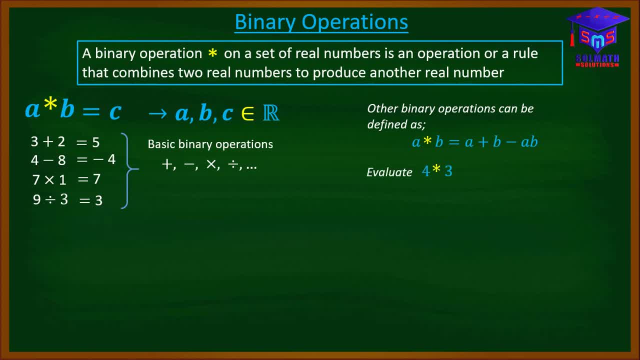 So you may be asked to use this definition to evaluate 4 star 3.. The only thing you have to do is that you relate the A to the 4 and then the B to the what 3.. Is that right, Good? 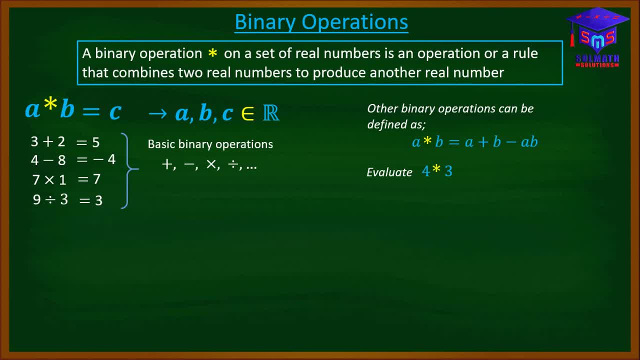 And so, wherever I will find A in a definition, we are going to put what 4.. And then, wherever I will find B, we are going to put what 3.. And so this will be given as 4 plus 3 minus what 4 times 3.. 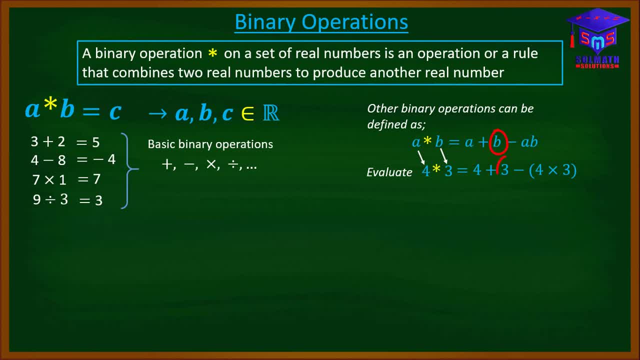 We just replace this A with what 4.. And then that B with what 3.. And then the AB over here with what 4 and 3.. So you simplify this further to get what Negative 5.. And so you see that we have combined these two real numbers- 4 and 3, with the operation star. 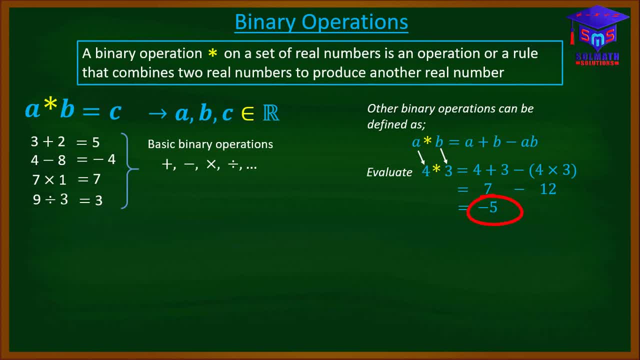 to produce another element, what 5,, which is also a real number, And so our binary operation in this case is: what Star Alright. and so other binary operations: star, this triangle: O plus, O dot, O times, O minus. 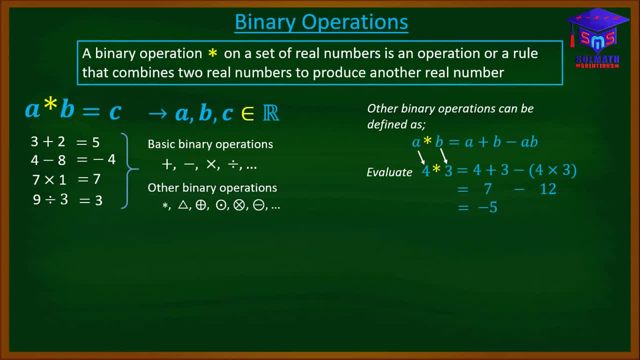 and many other advanced binary operations can be used. So instead of the star over here, you may find something like these ones. Alright, let's take an example. A binary operation, star, is defined as what A star B is equal to 4A minus B. 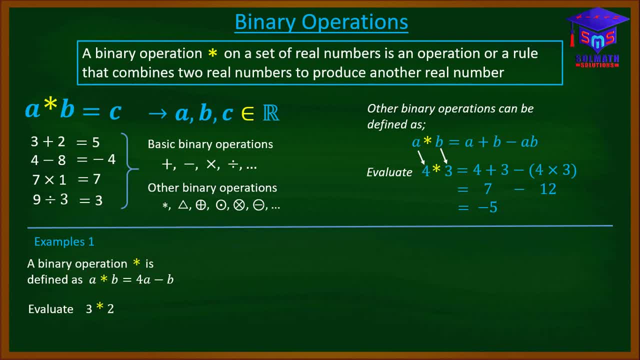 Evaluate 3 star 2.. Okay, so we have a binary operation defined for us And then we are asked to use that to evaluate what 3 star 2.. So get down your defined operation nicely. So we are going to relate the A to the 3 and then the B to what 2.. 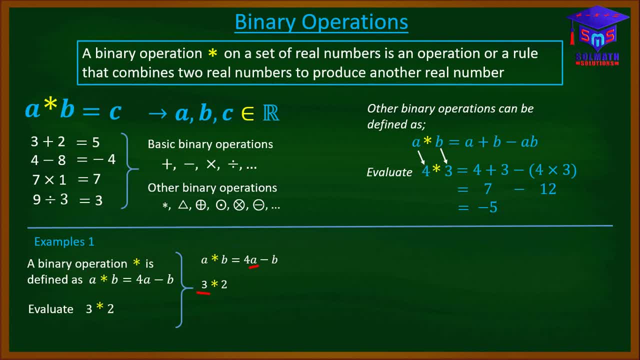 So, wherever we find A in a definition, we are going to put what 3.. And then, wherever we find B, we are going to put what 2.. That's right. And then, in simple terms, what this definition means is that multiply the A with 4 and then subtract what The B. 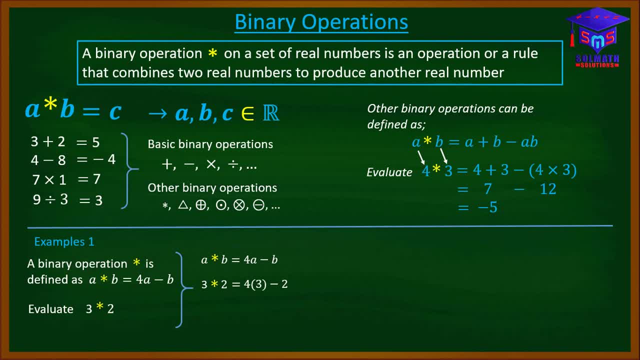 Okay, so after substitution we get something like this, which simplifies to give us 12 minus 2, and then that is what 10.. So you realize that we have combined these two real numbers, 3 and 2, using the binary operation. what Star. 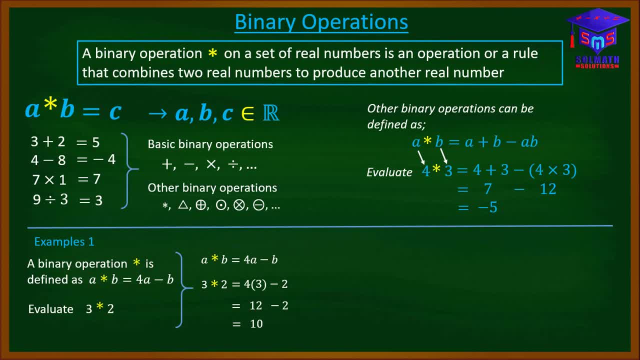 to produce another element. what 10.. So the binary operation is: what A star, The star we have over here. Alright, let's take a look at another example. If x operation y is equal to x squared plus 2y minus xy, evaluate 5 operation 3.. 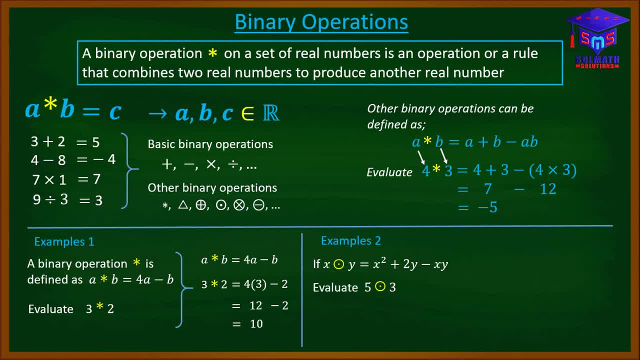 The operation is circle dot. okay, Alright, this binary operation defined for us. the only thing it means is that you square the x and then add 2 times the y and then subtract the product of what x and y. Very simple. 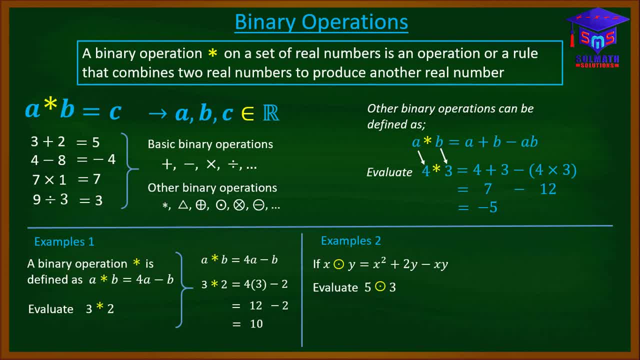 So in evaluation we are going to relate the x to 5 and then the y to what 3.. Okay, so, alright, So you put down the definition nicely, and then this is what we are supposed to evaluate. So we are going to relate the x to the 5 and then the y to what 3.. 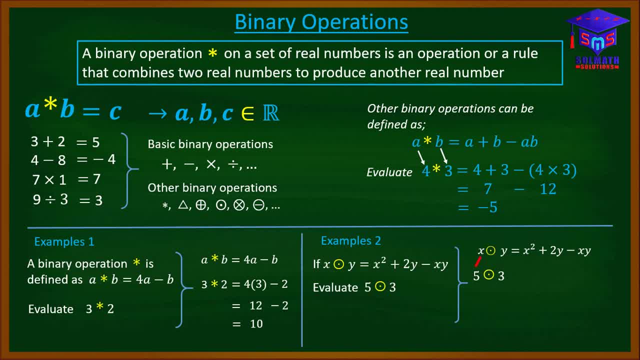 So, wherever I will find x in the definition, we are going to put 5.. And then, wherever I will find y, we are going to put what? 3.. Okay, Alright, so this is giving us 5 squared plus 2.. 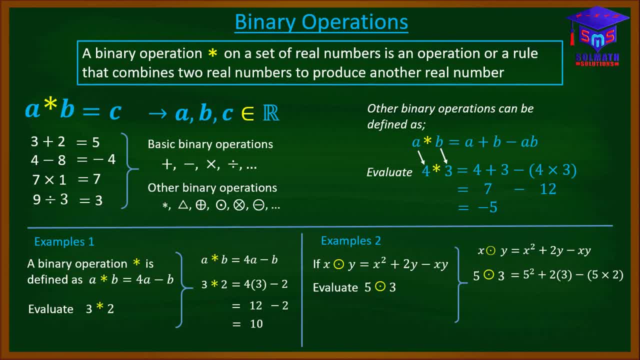 Plus 2 times 3, minus 5 times 2.. Okay, And then you simplify it nicely, and then you are getting what? 21.. So we have combined these two real numbers, 5 and then 3, using the binary operation circle dot to produce another real number, 21.. 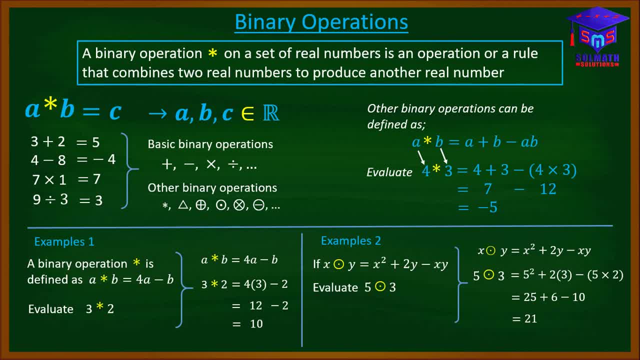 Okay, So that is the whole idea of binary operation. It is simply an operation or a rule that combines two real numbers to produce another real number. Okay, And that binary operation can be addition, subtraction, multiplication, division or any other defined binary operation. 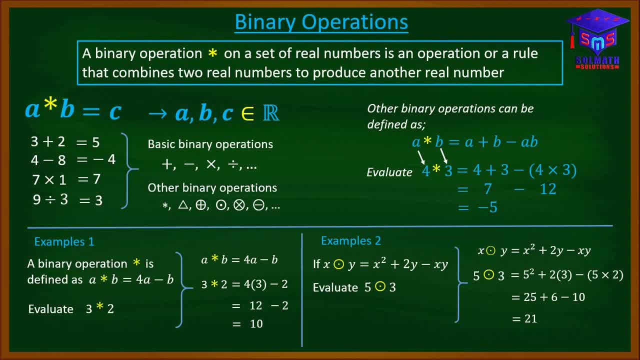 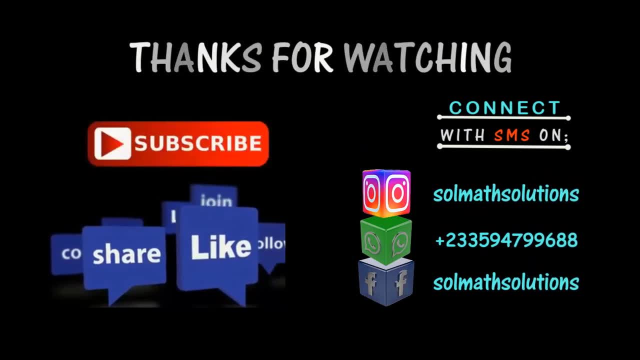 Alright. In the next session we will look at closure. Stay tuned, Thank you.